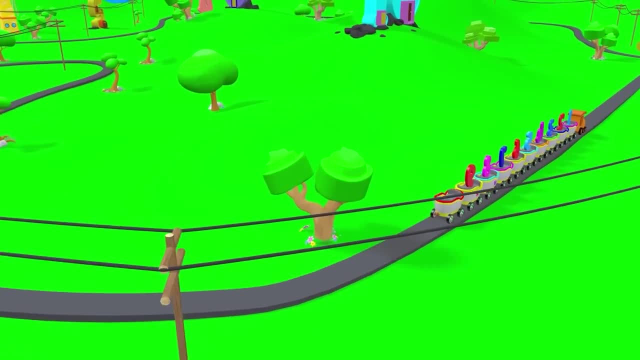 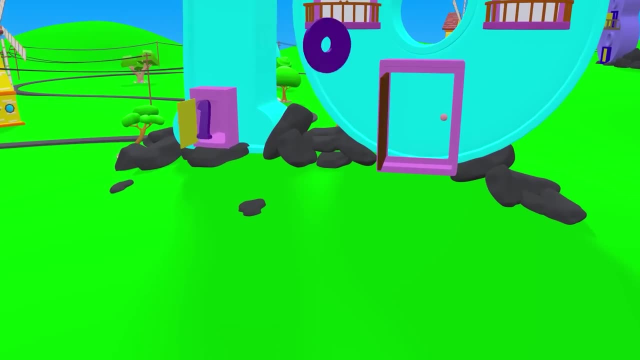 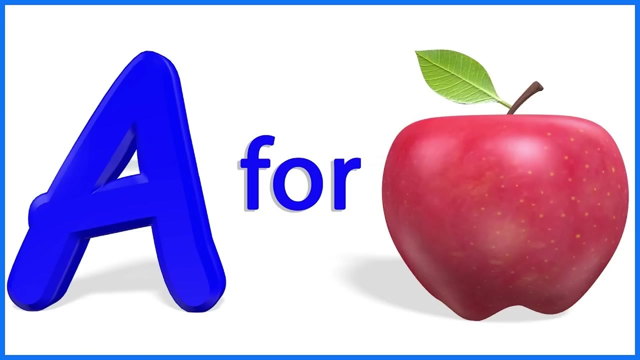 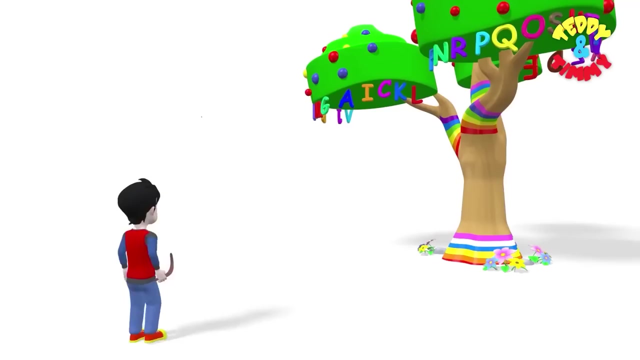 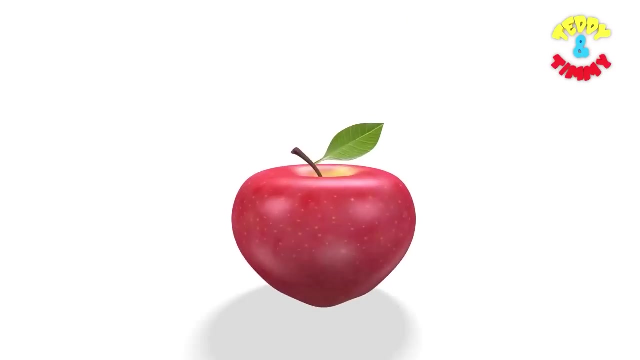 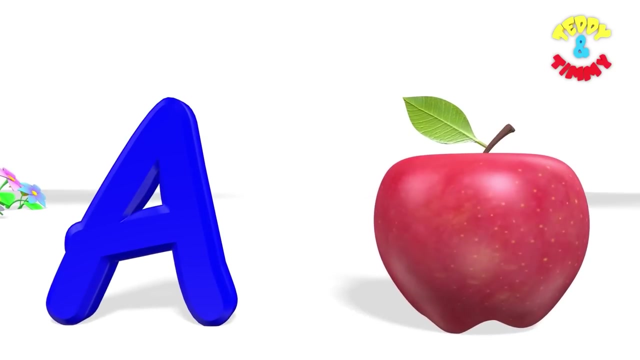 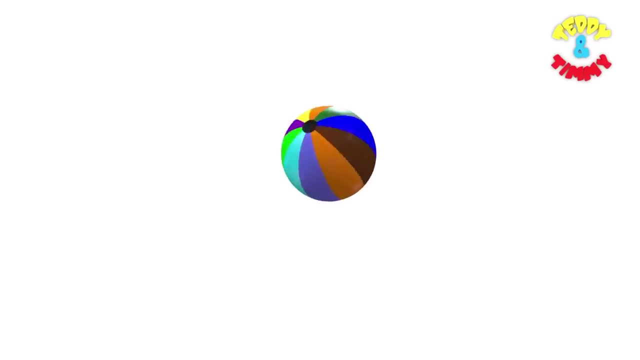 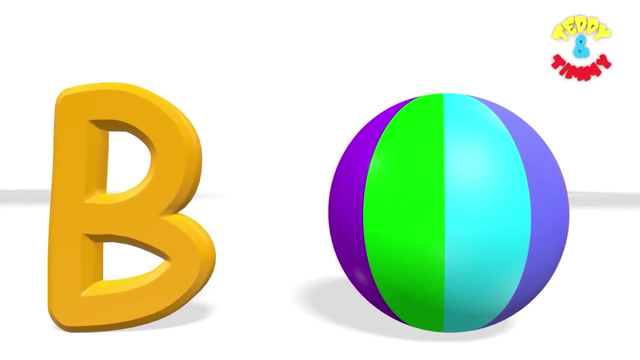 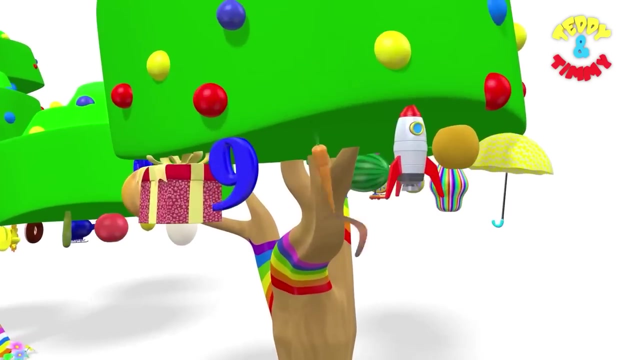 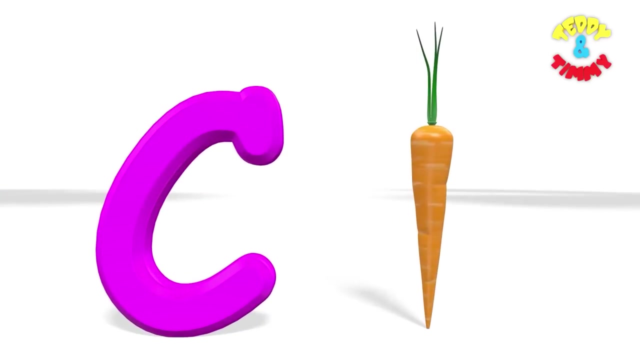 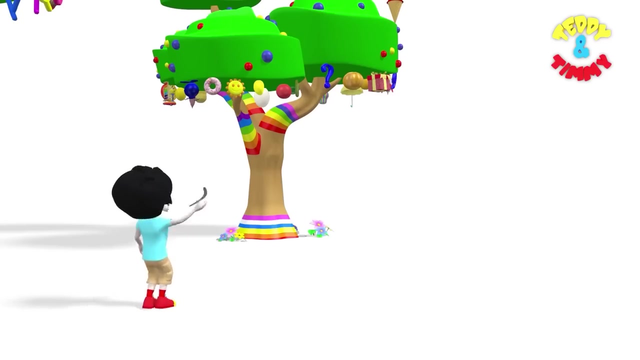 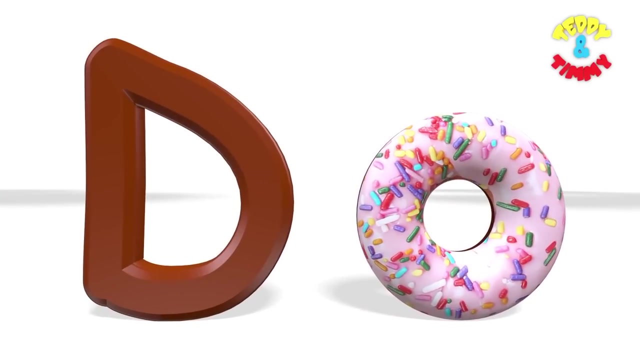 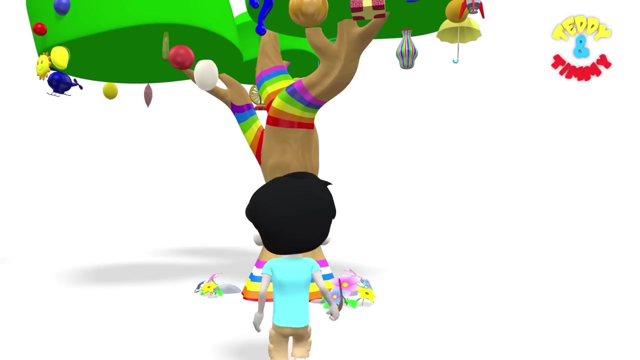 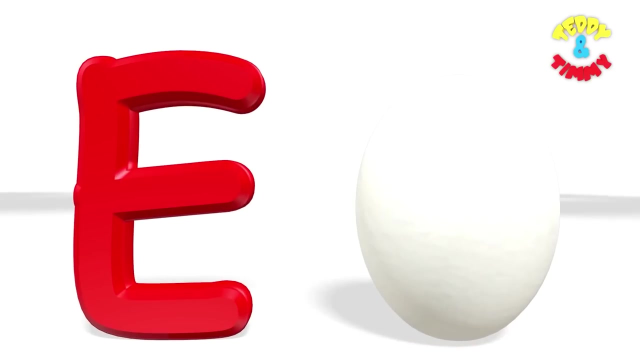 Thirteen, Ten, Eight, Twelve: Apple A for Apple B, Ball B for Ball C, Carrot C for Carrot D, Donut D for Donut E, Egg E for Egg. 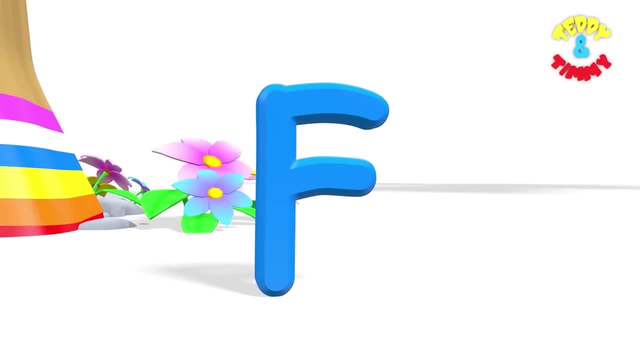 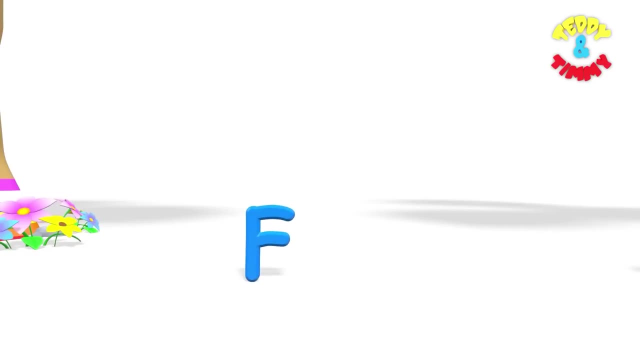 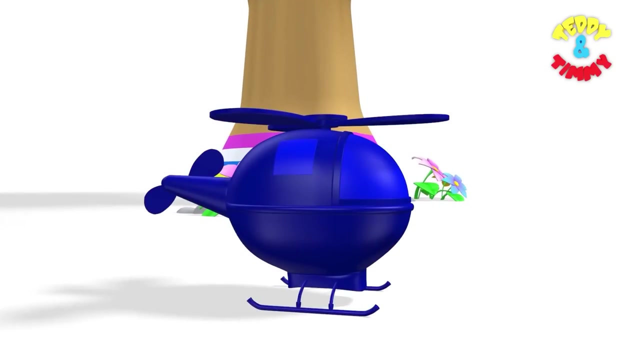 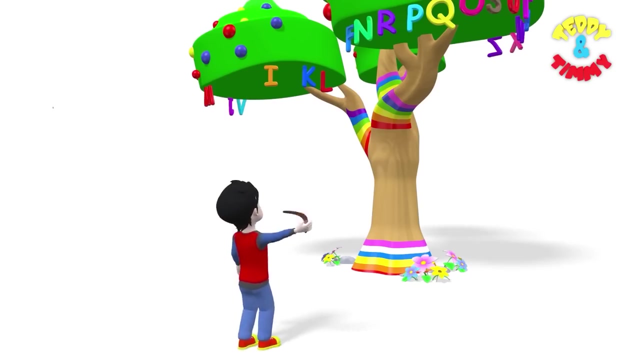 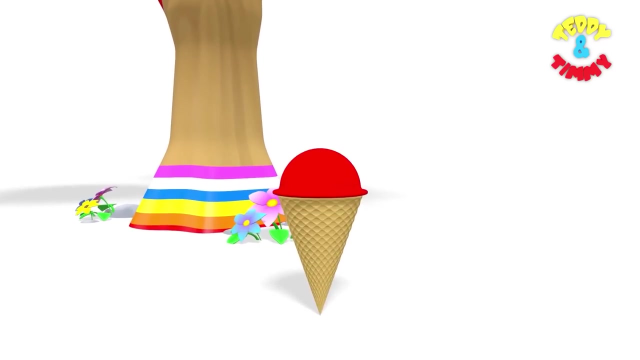 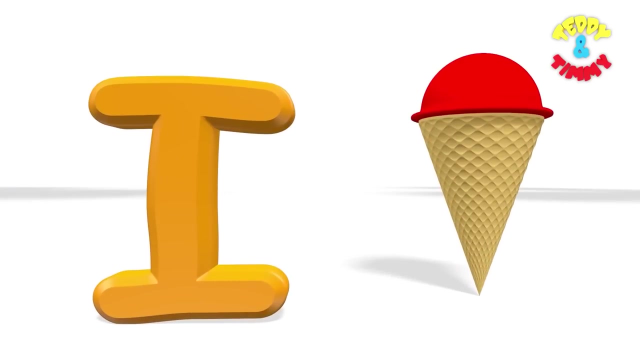 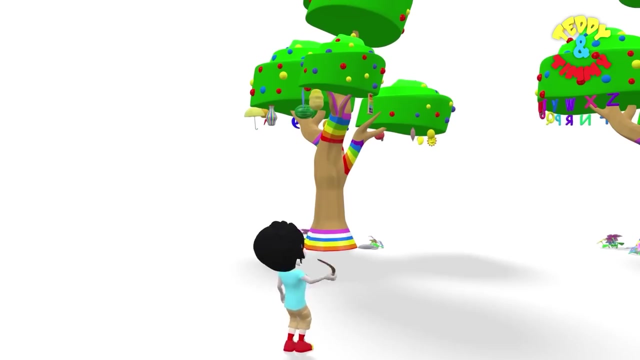 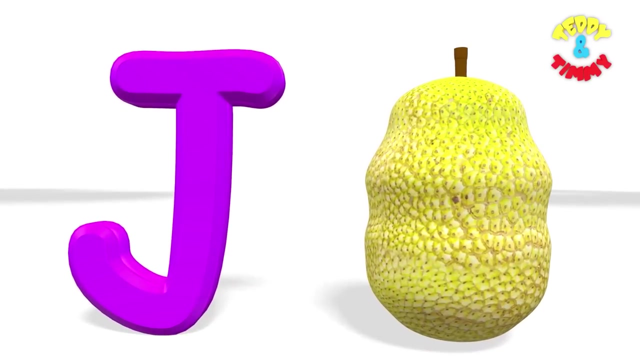 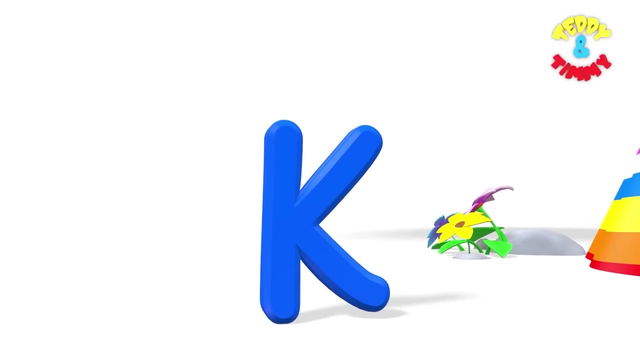 F. Fan F for Fan G, Gift G for Gift H. Helicopter H for Helicopter I. Ice Cream- I for Ice Cream J. Jackfruit J for Jackfruit, K, Kite. 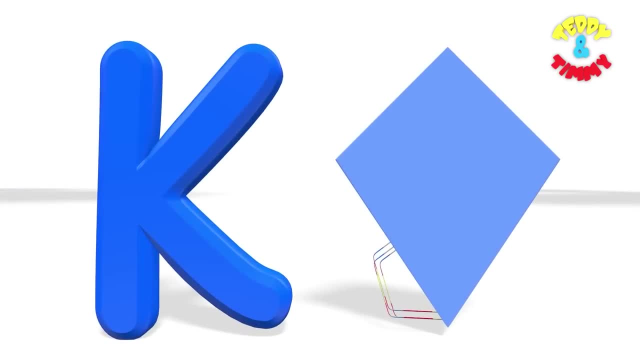 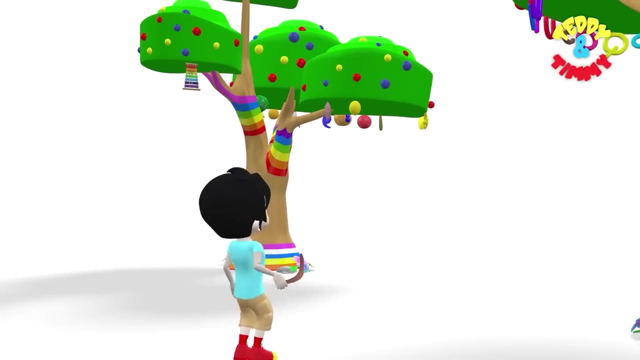 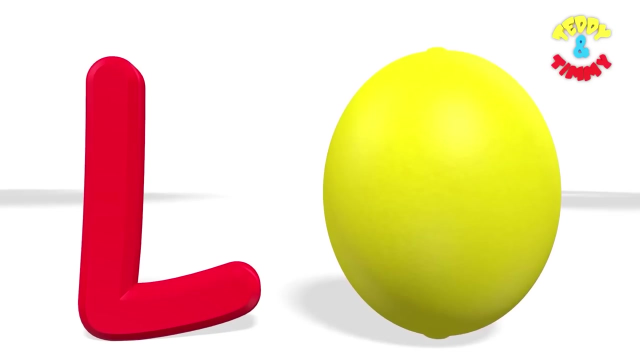 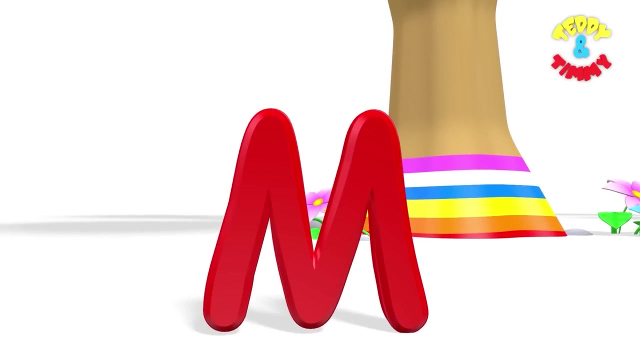 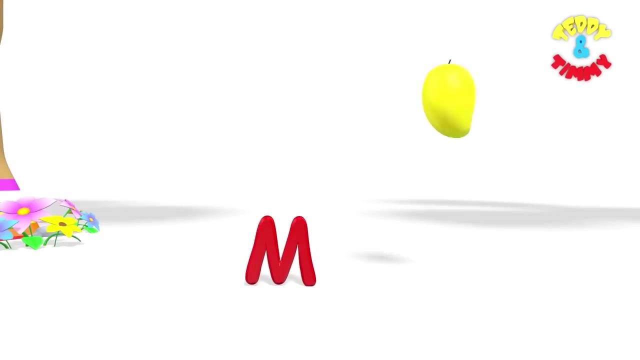 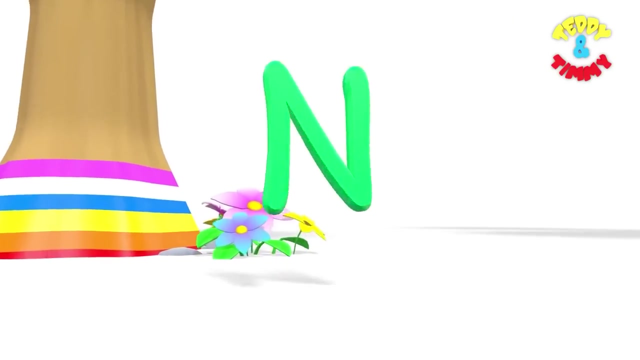 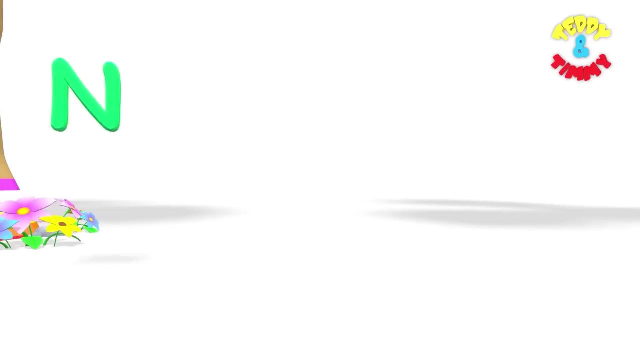 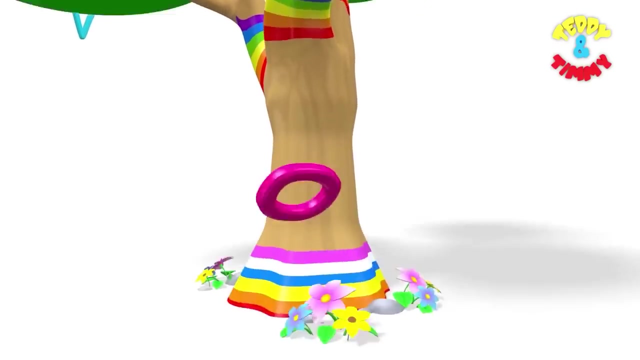 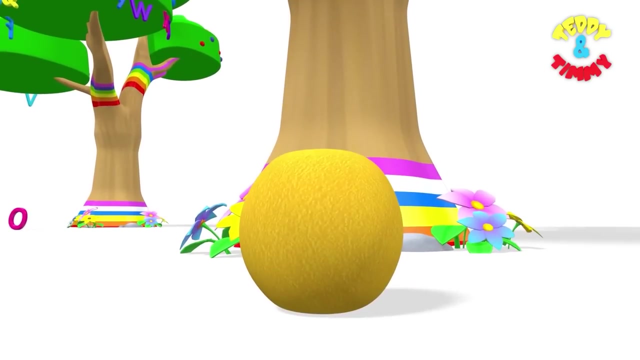 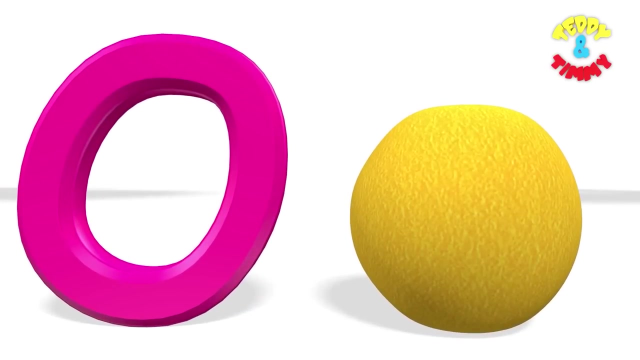 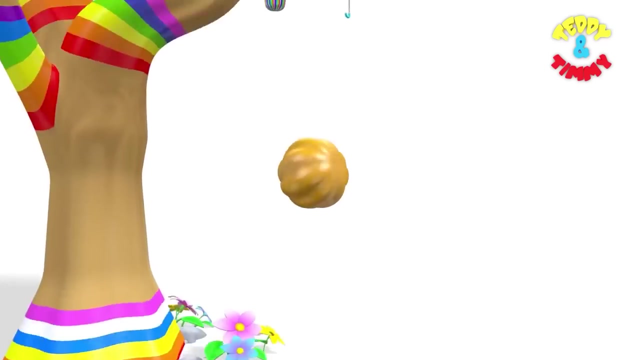 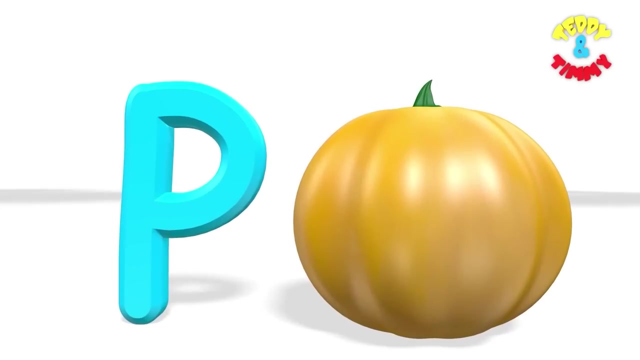 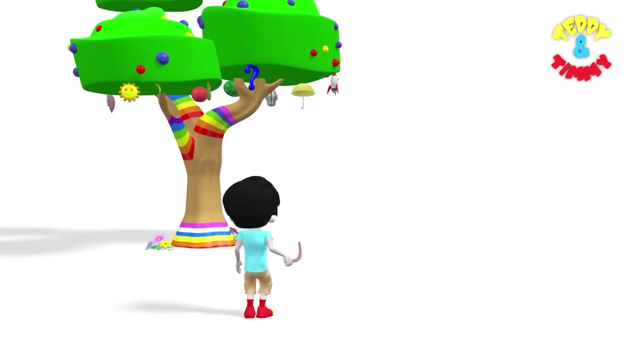 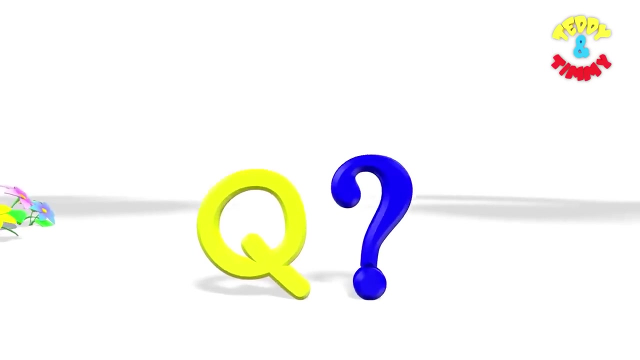 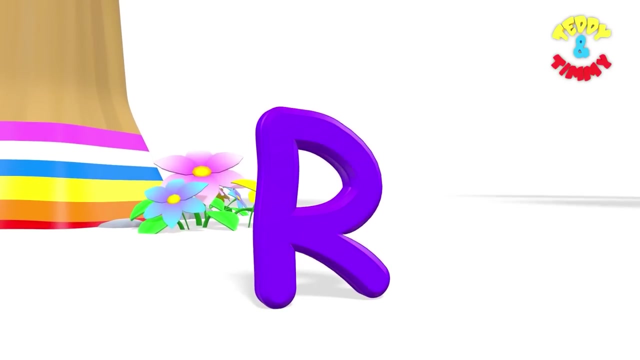 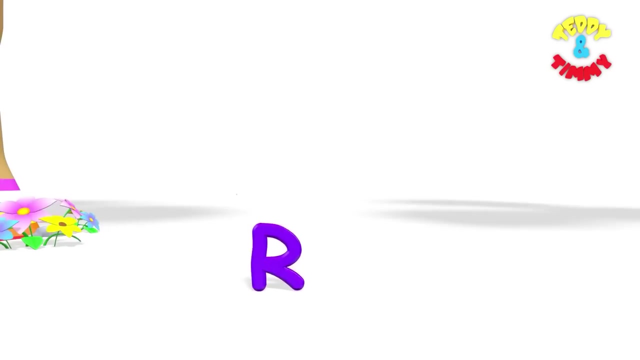 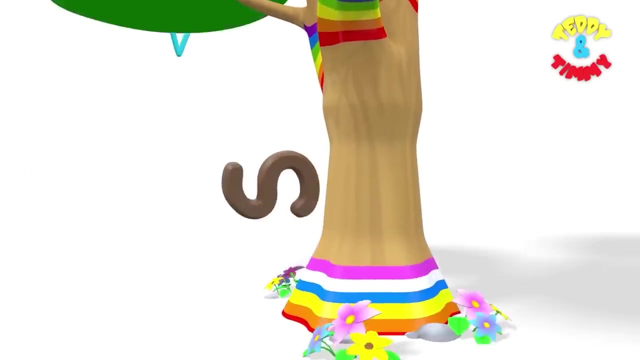 K for Kite L. Lemon L for Lemon, J for Lemon M. Mango M for Mango N. Nine N for Nine O. Orange O for Orange P. Pumpkin P for Pumpkin. Q for Pumpkin Q. Question Q for Question R. Rocket R for Rocket S. 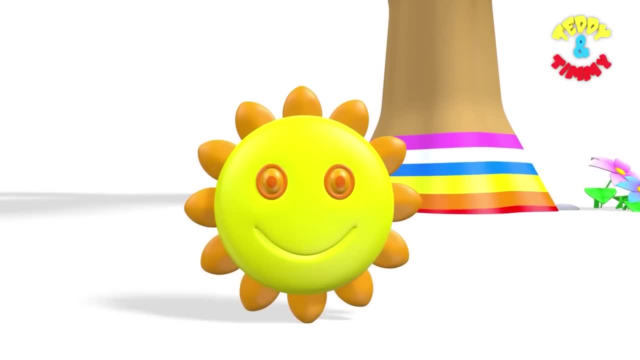 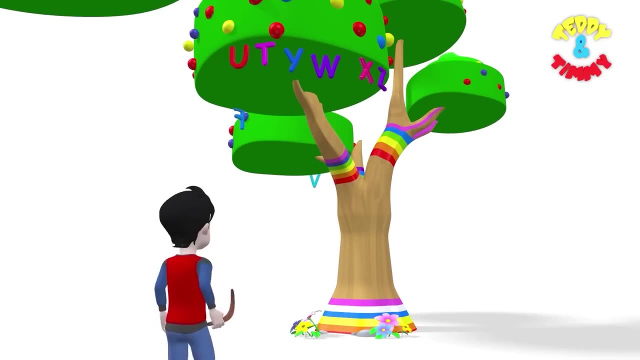 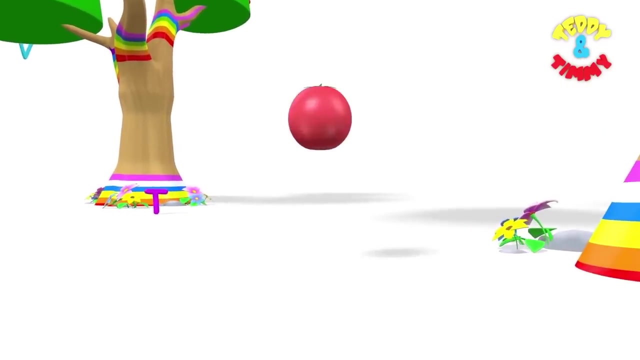 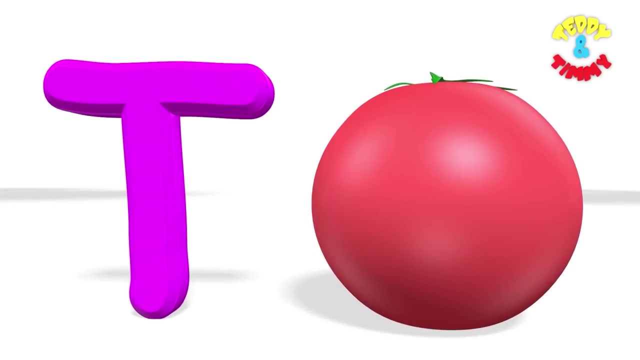 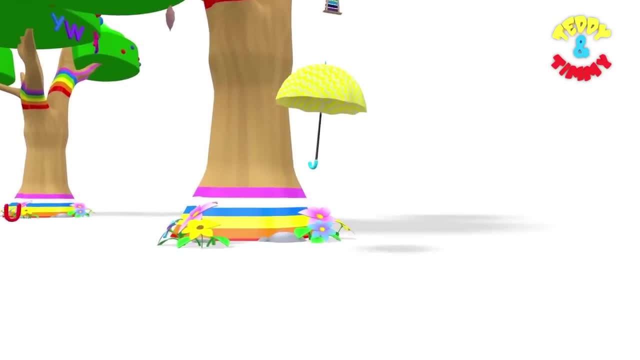 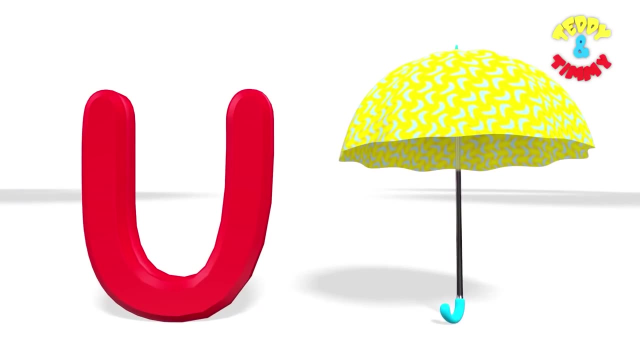 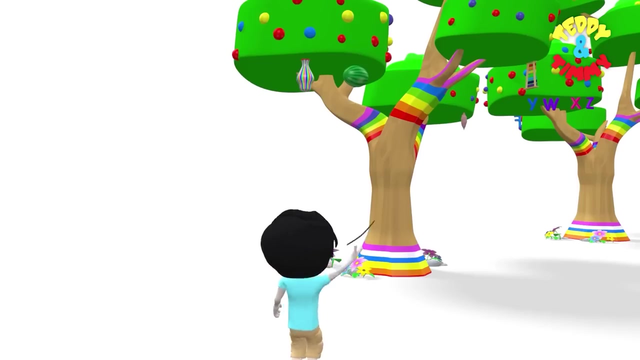 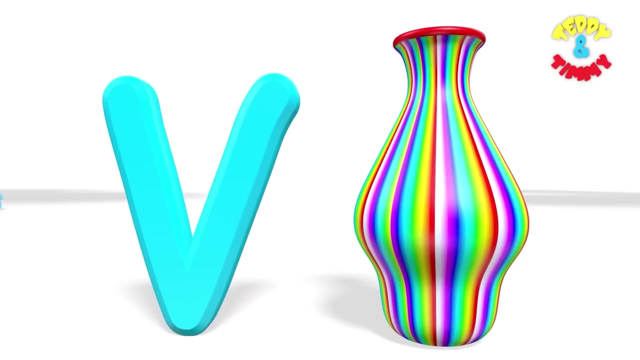 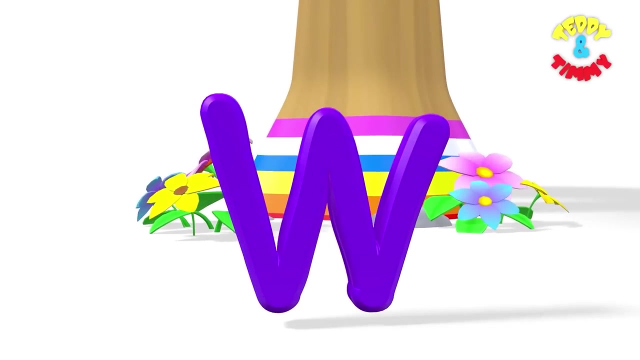 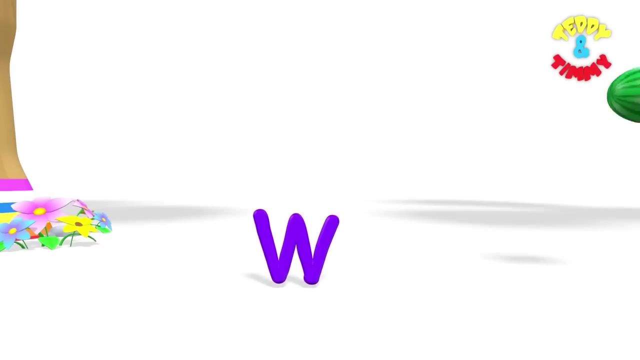 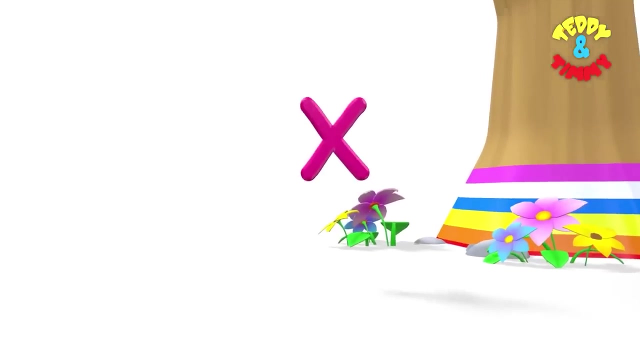 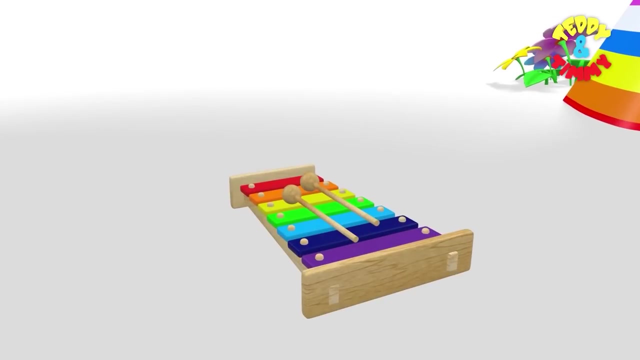 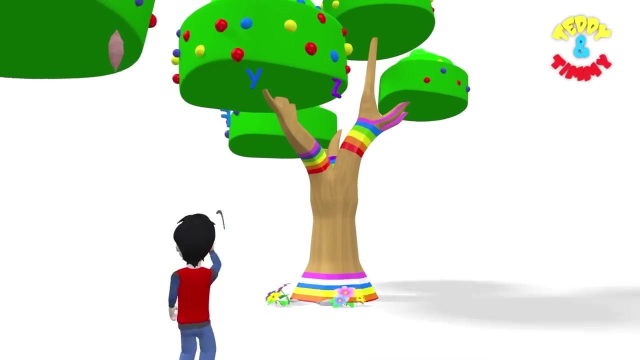 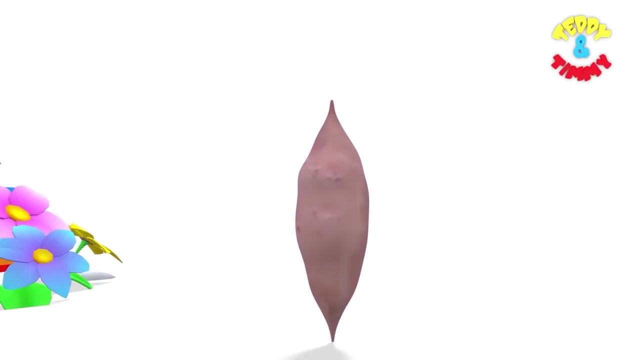 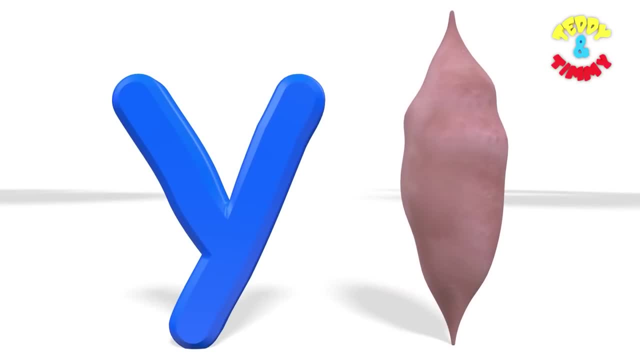 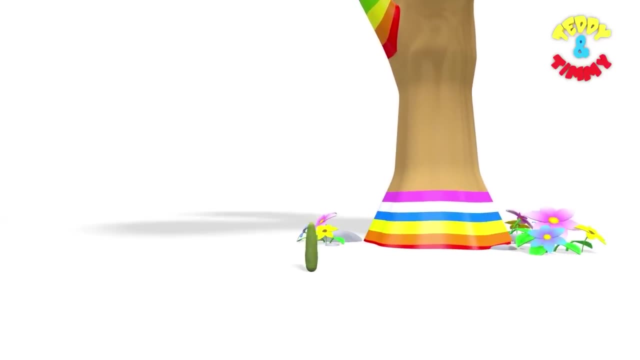 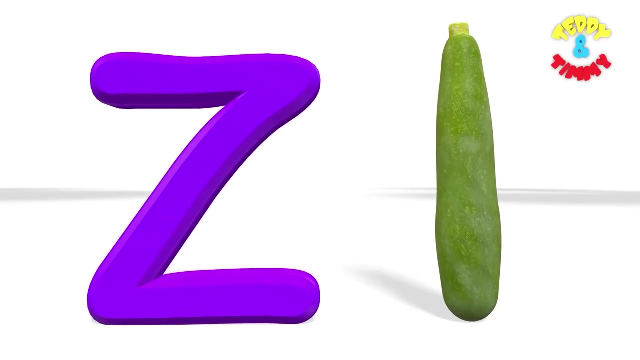 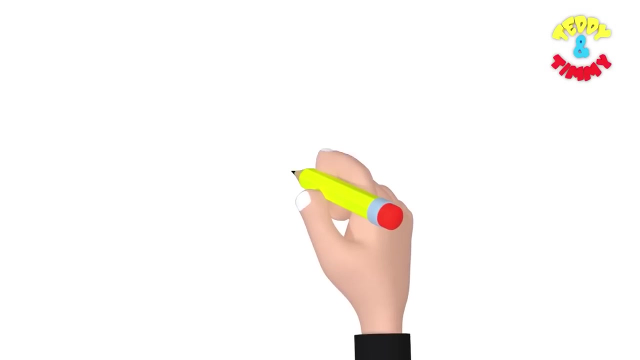 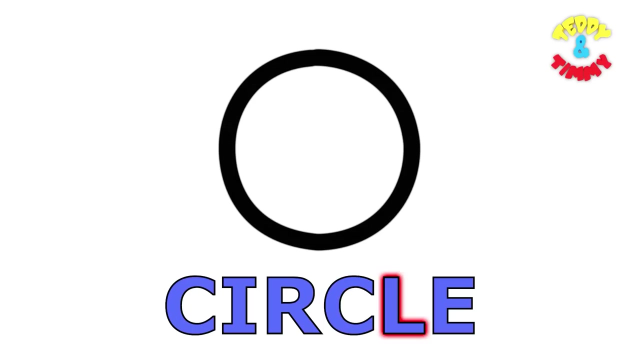 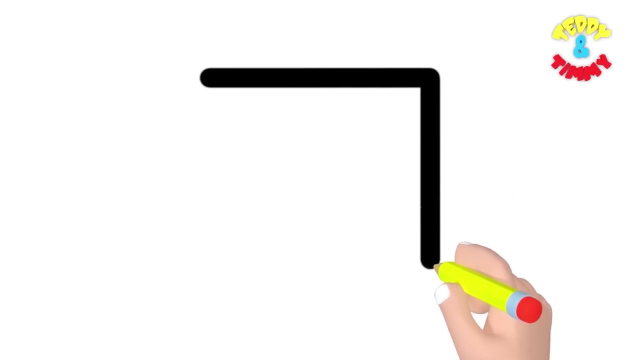 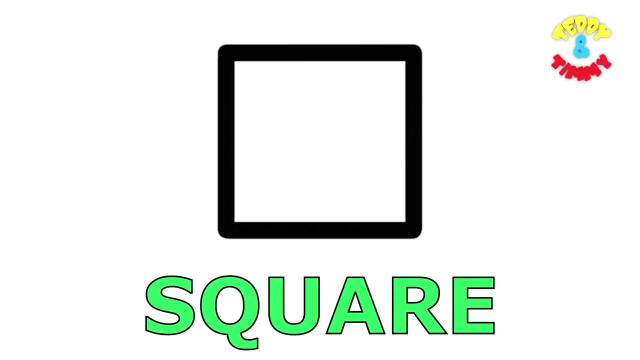 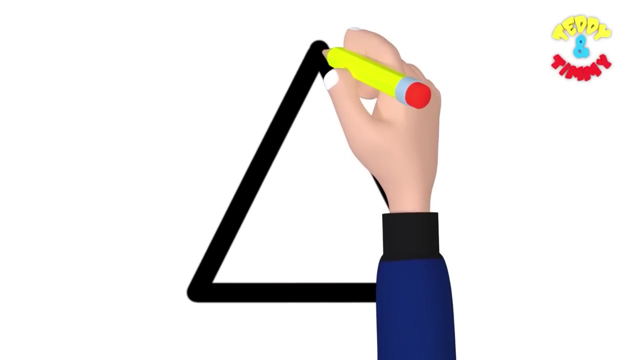 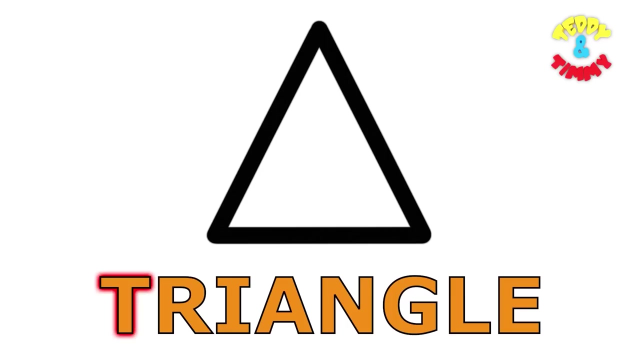 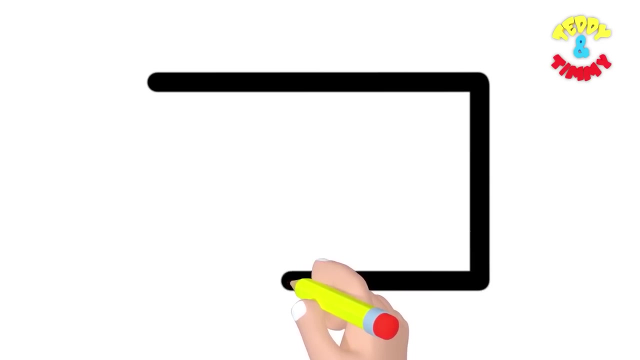 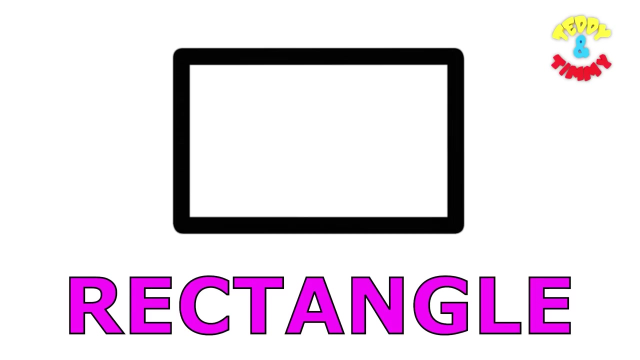 Y for Yem Z Zucchini Z for Zucchini Circle. C-I-R-C-L-E Circle Square. S-Q-U-A-R-E Square. Triangle- Triangle. T-R-I-A-N-G-L-E Triangle Rectangle- Rectangle. Rectangle. R-E-C-T-A-N-G-L-E Rectangle. 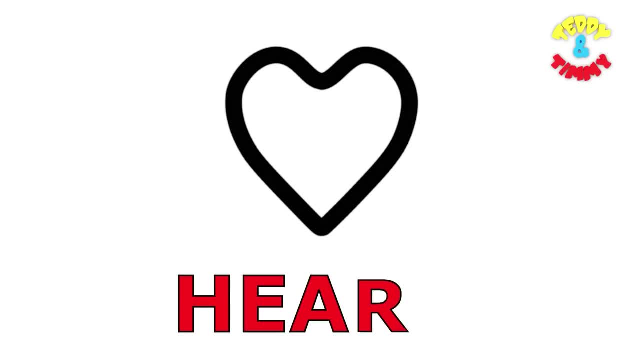 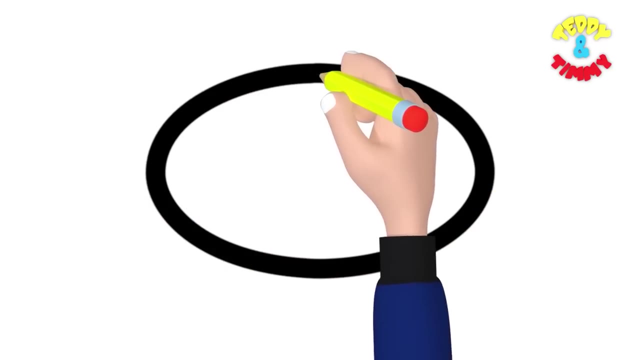 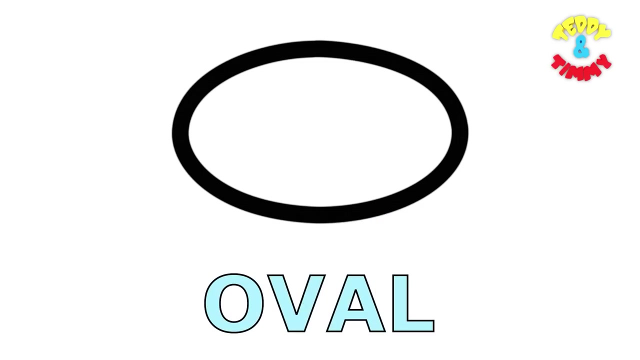 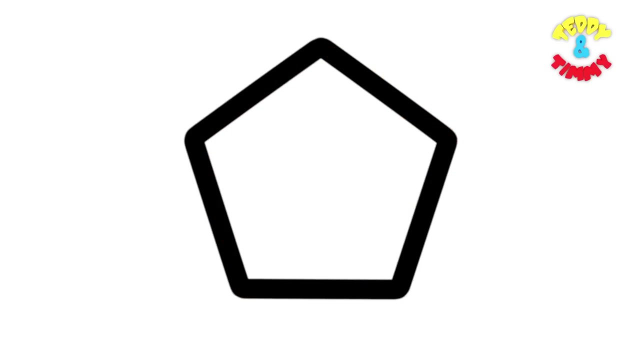 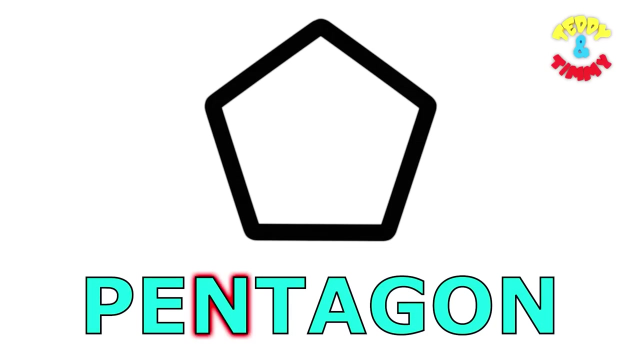 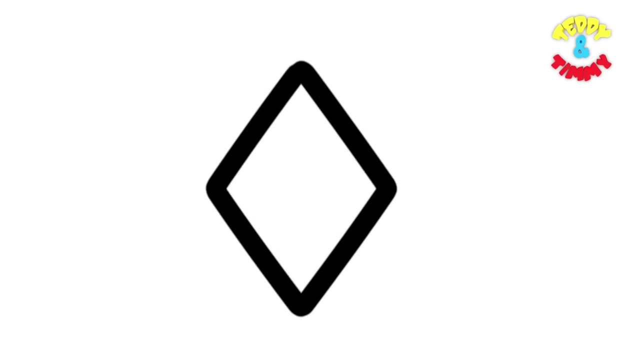 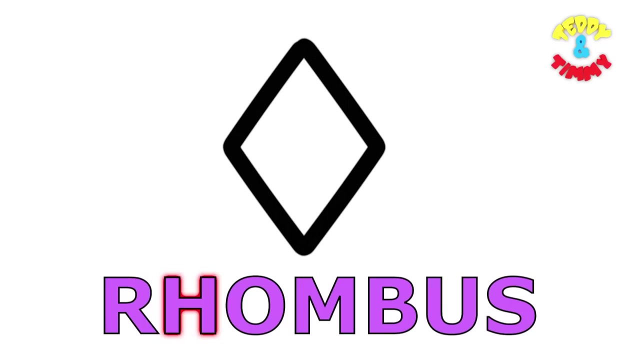 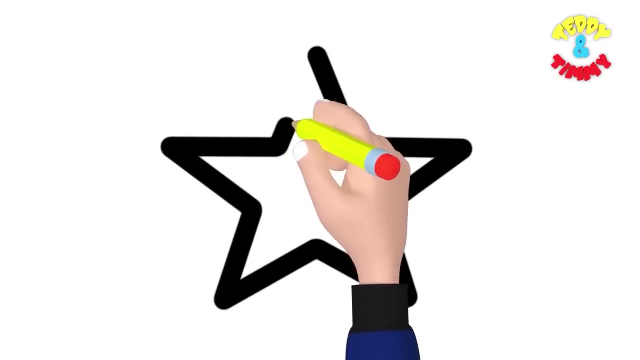 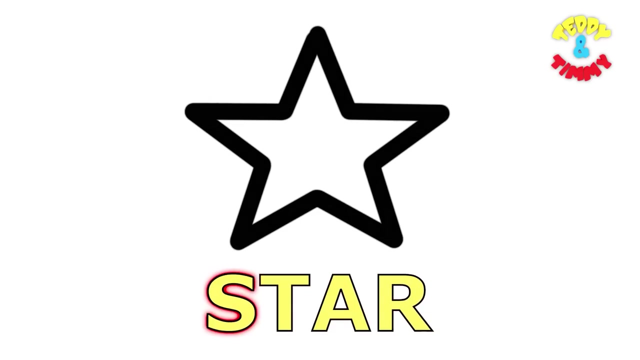 Heart H-E-A-R-E R D Heart. Oval O V A L Oval. PENTAGON. P E N T A G O N. PENTAGON. Rhombus R H O M B U S. Rhombus Star S T A R. Star S T R. 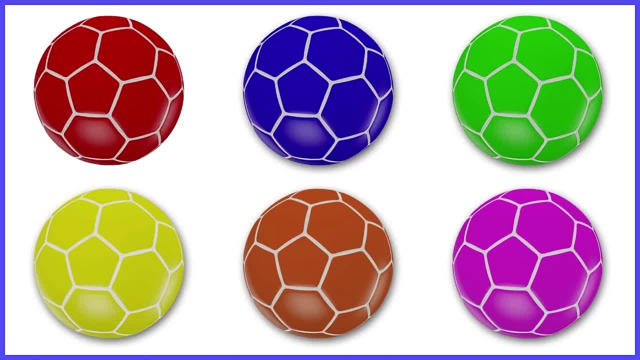 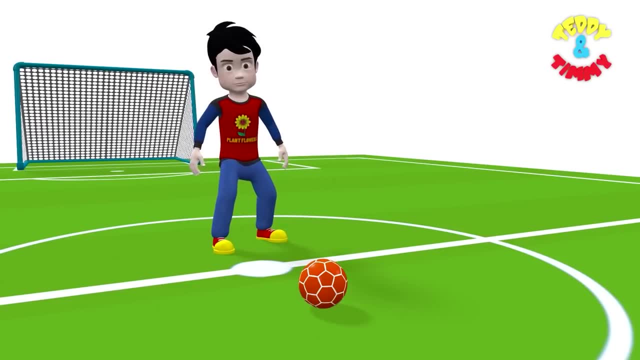 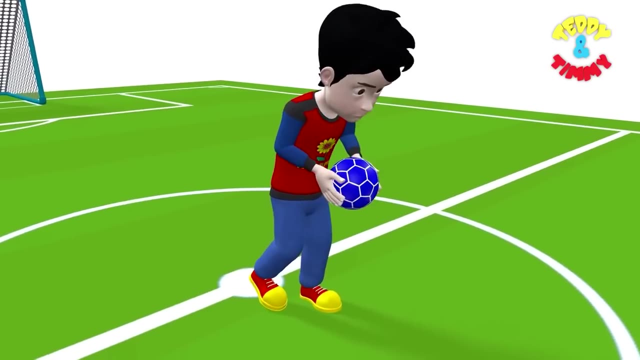 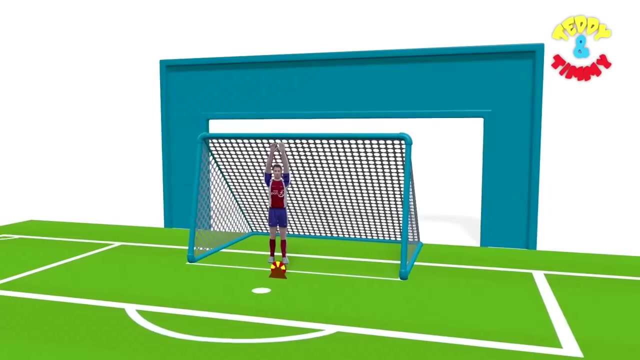 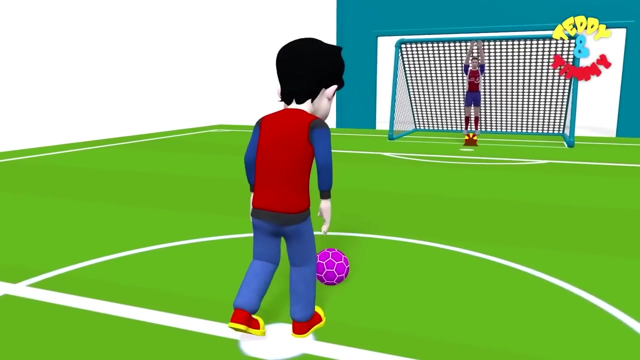 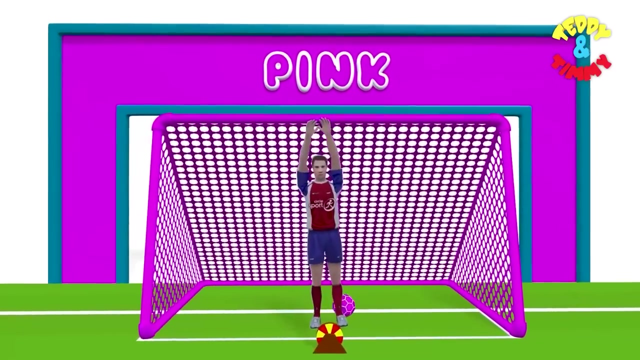 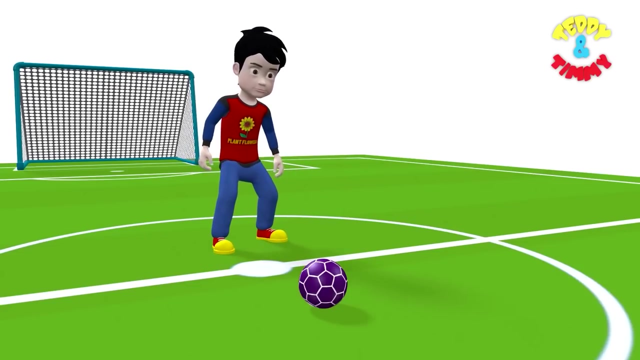 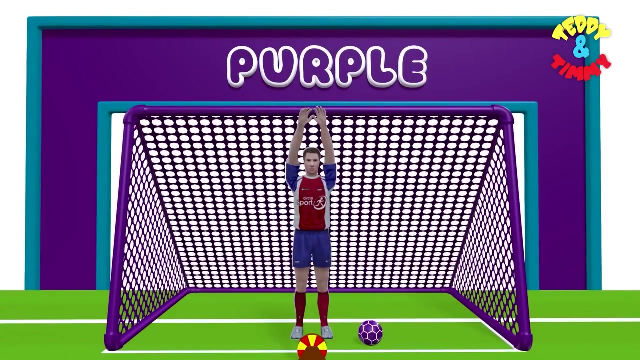 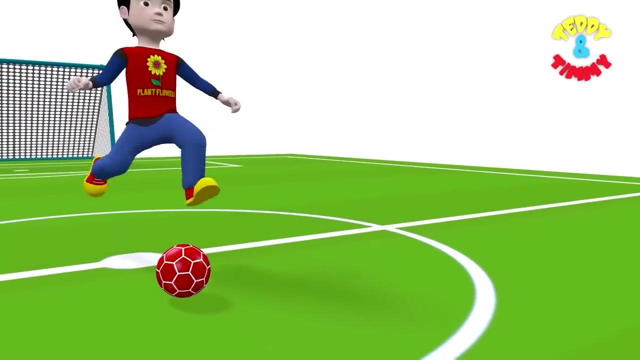 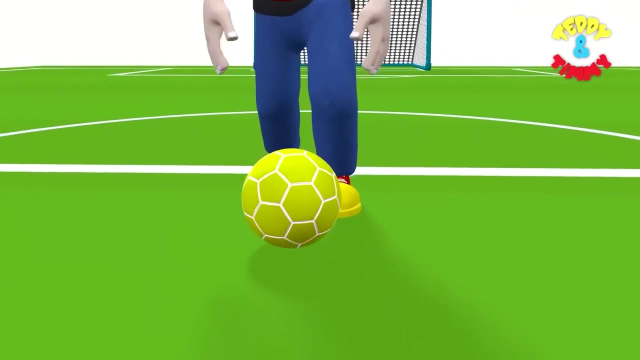 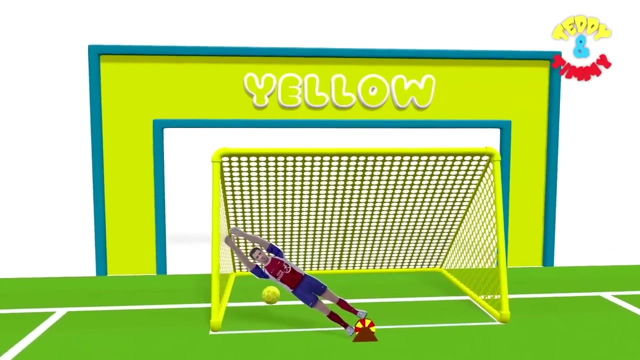 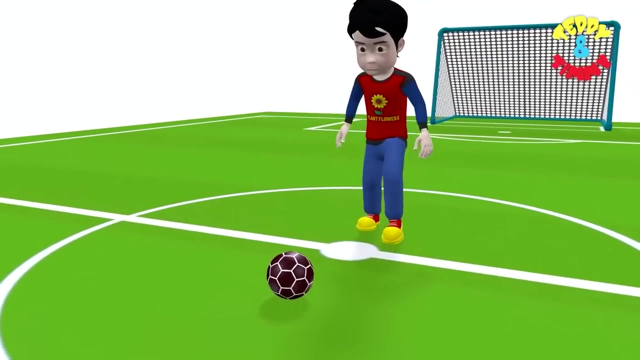 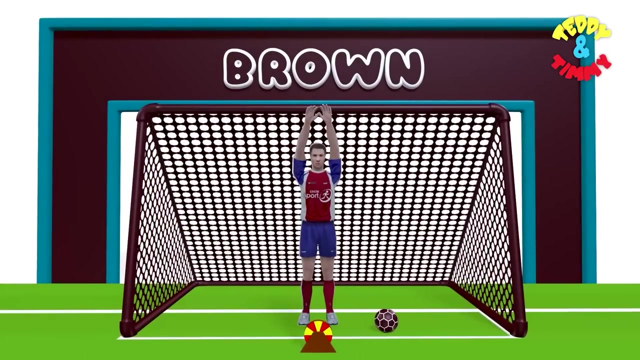 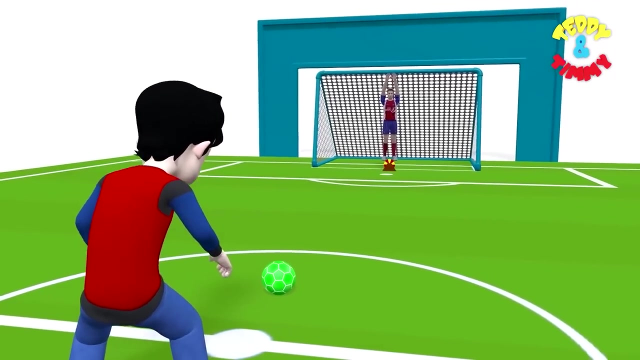 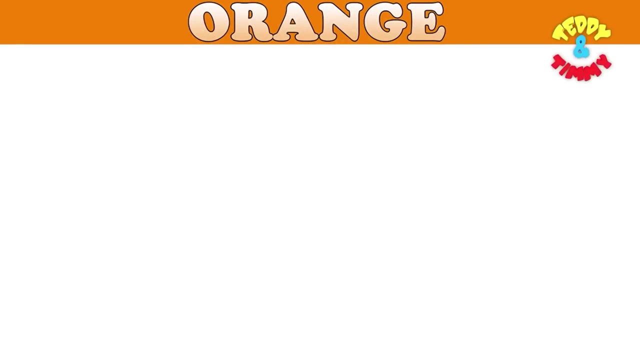 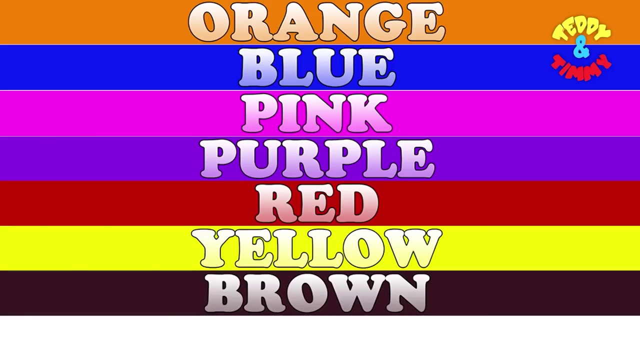 S T R. Orange, Orange, Blue, Pink, Purple, Blue, Red, Yellow, Brown, Green, Orange, Blue, Pink, Purple, Red, Yellow.